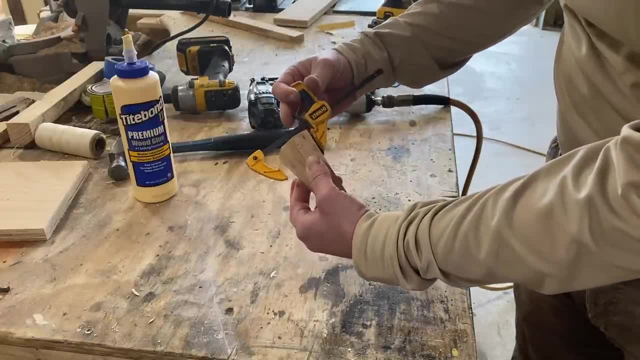 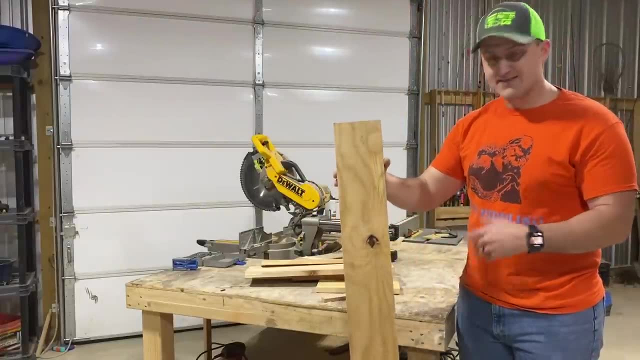 If you've ever worked with plywood, you probably notice that you have these long skinny strips left over- At least I do, anyways- And it seems like you can't do anything with a piece this size. Try making your own track saw with that. If you have a circular saw, this actually cuts up big. 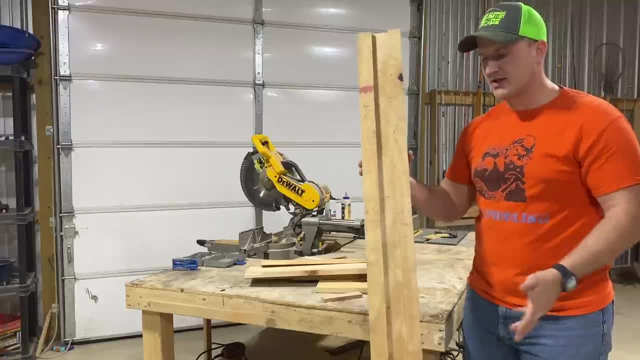 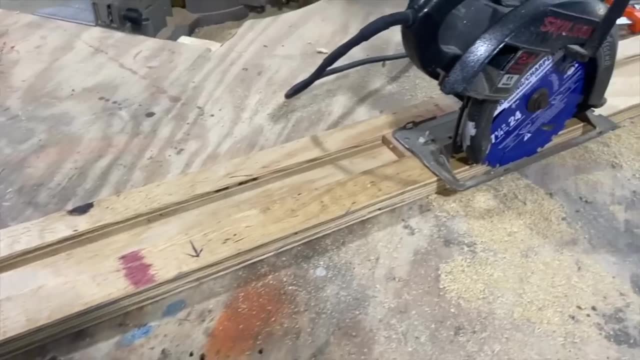 pieces of plywood a lot easier than a table saw will, And this is a super simple project. This particular scrap wood project only takes about an hour or so, and it's a lot of fun to build Now. if you've ever worked with plywood, you'll probably notice that you have these long, skinny 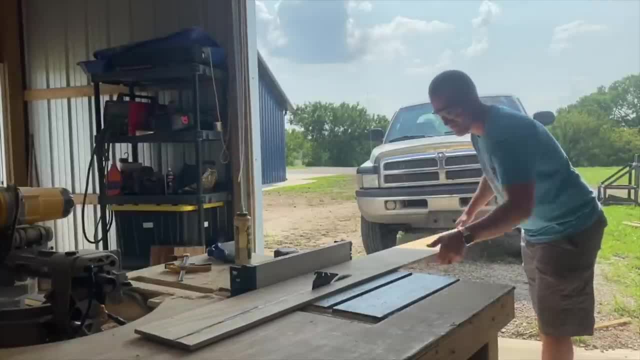 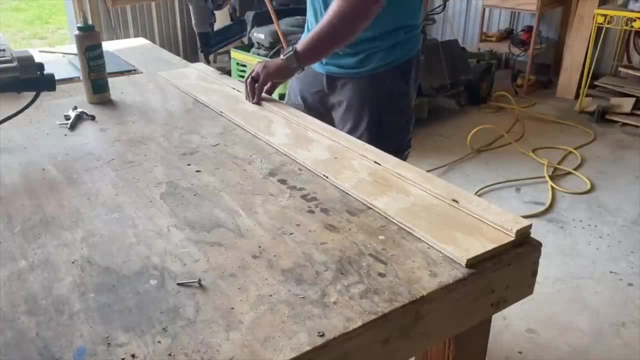 strips left over. At least I do. anyways, It is ideal to build these using a table saw, but if you don't have one, a circular saw will work as well, And once you're finished with this project, this is a nice tool to have, because it's really nice to be able to cut plywood straight. 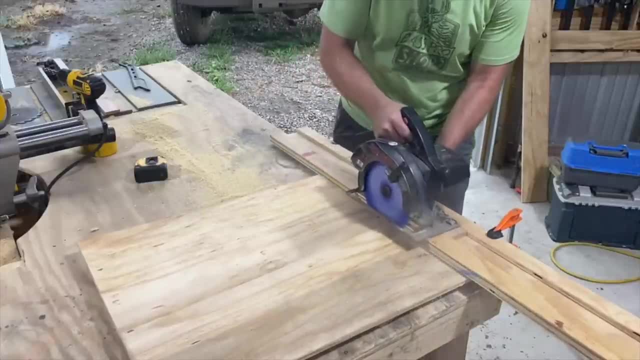 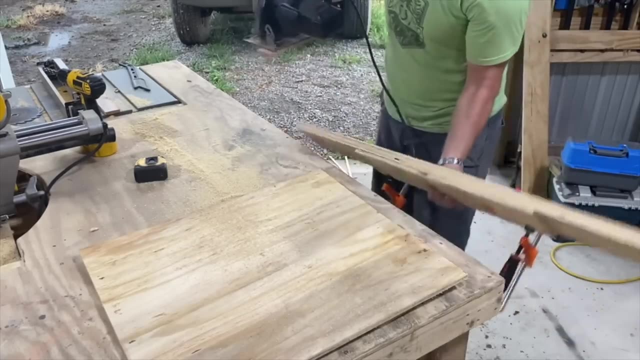 And I personally think, when you're cutting big pieces of plywood, this is a lot easier to deal with than the circular saw. But don't take my word for it. Try making one for yourself. You might as well do something with that extra plywood. Now I don't want to toot my own horn. 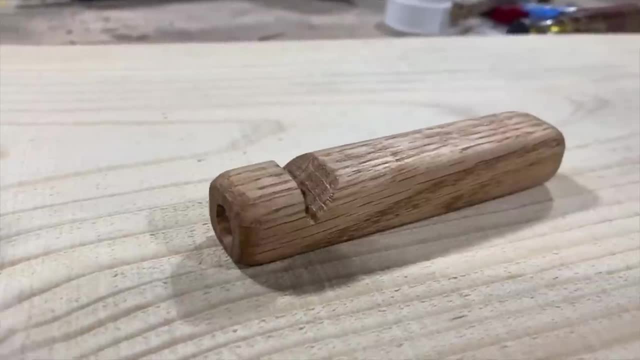 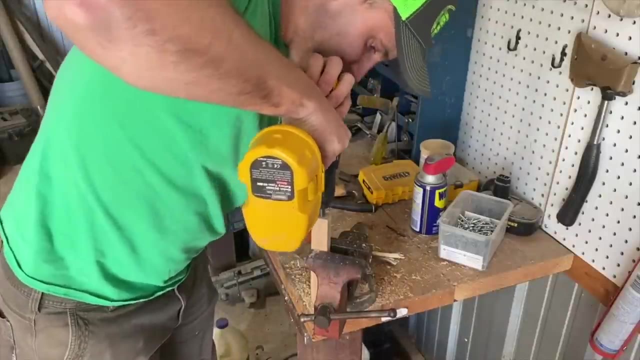 but another easy scrap wood project that you might like is a simple toy whistle. This one's super easy to build and it's really quick. I had a lot of fun making this project and I actually had a few failed attempts before I made this one that actually worked. 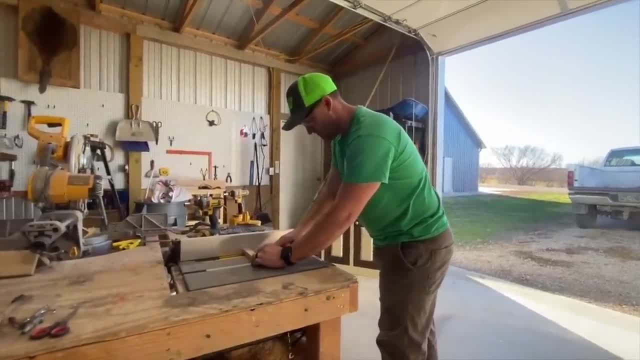 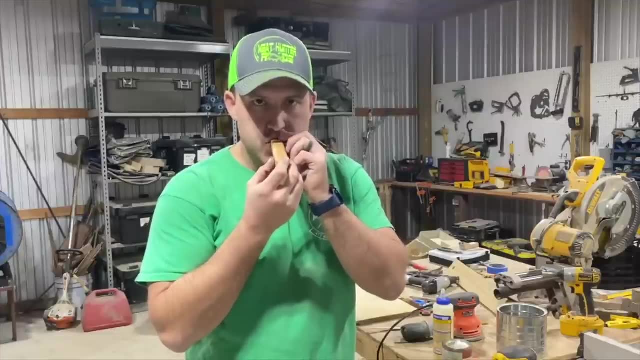 One of my favorite things about YouTube is that you can learn how to do just about anything on there. With this little scrap wood project, not only did I learn something new, but I also had a little gift to give to a friend. Worked pretty good, You have to admit, this is kind of a cool. 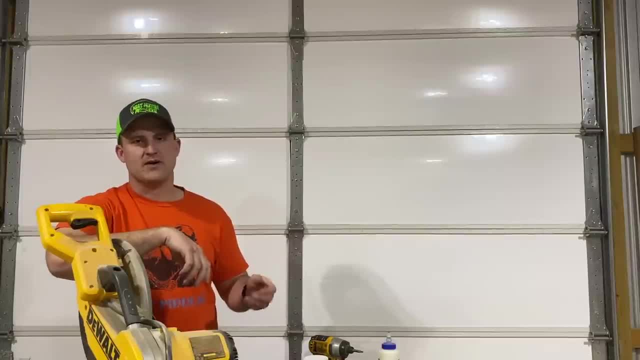 little project. Only about a week after I built that whistle, my brother-in-law shot me a text and said that he could toot louder than me, so I decided to do it myself. I'm going to show you how to do it. I'm going to show you how to do it and I'm going to show you how to do it. 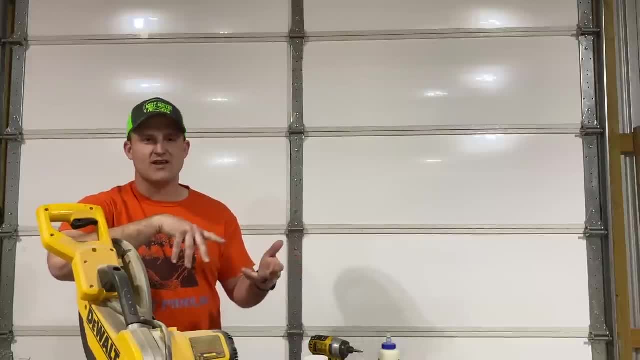 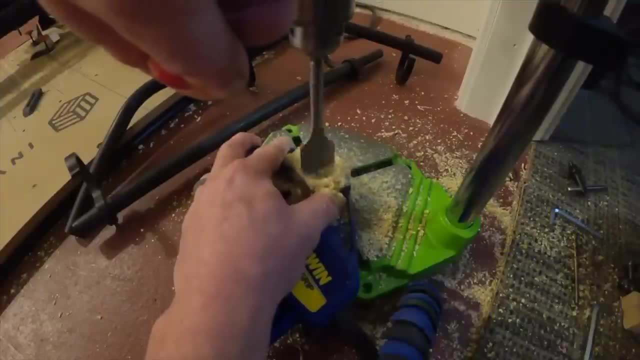 And so I was a little bit jealous, and what I mean by that is he built a train whistle and now I'm kind of jealous of his train whistle. I thought this was kind of a cool project because he used a scrap 2x2 to build it. 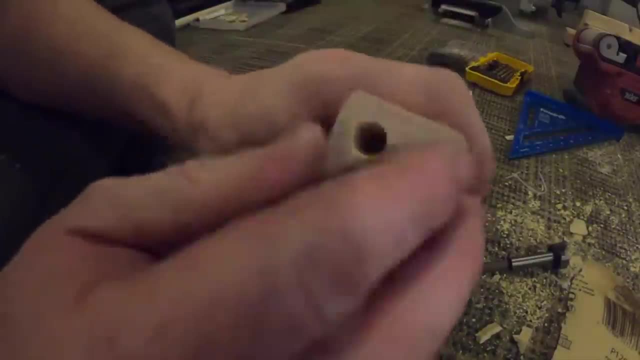 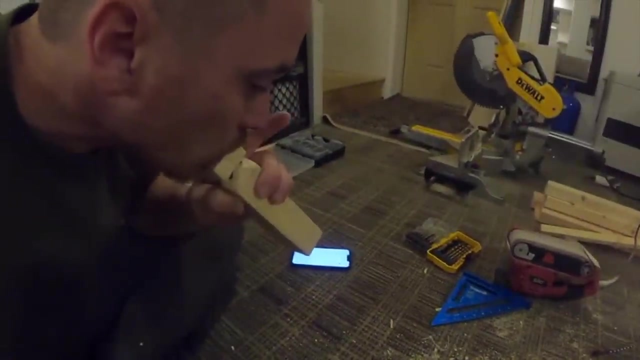 and now I kind of want to make one for myself. He actually made this look pretty simple and I think it turned out pretty cool, but don't tell him I said so. Here's a really simple scrap wood project that I use all the time. It's a half sheet. 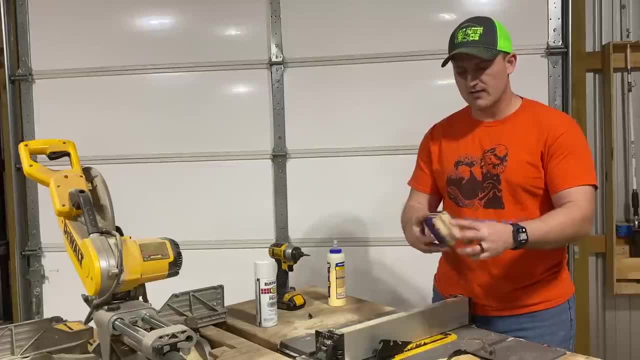 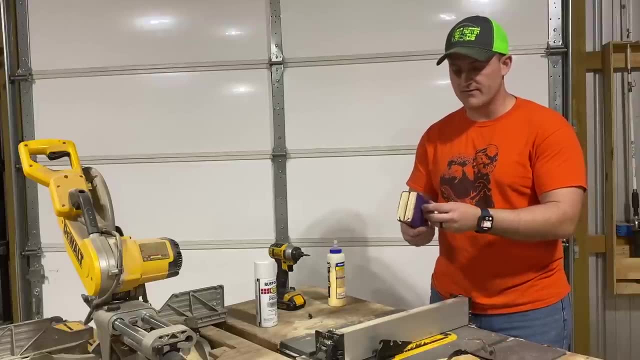 sanding block. This is a super easy project and it really doesn't take that much time to build. This thing comes in handy and I have a lot of sanding equipment, but I end up using this a lot for different things. To make one of these, you can use just about any scrap wood you have laying. 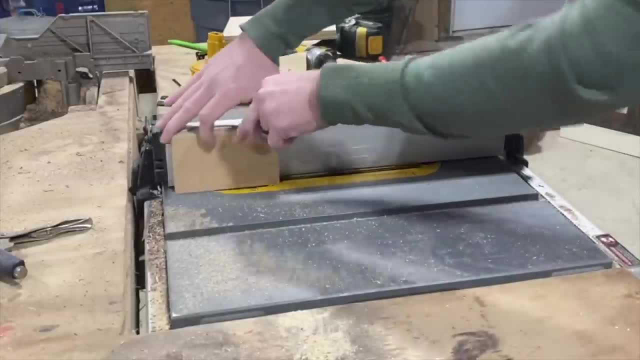 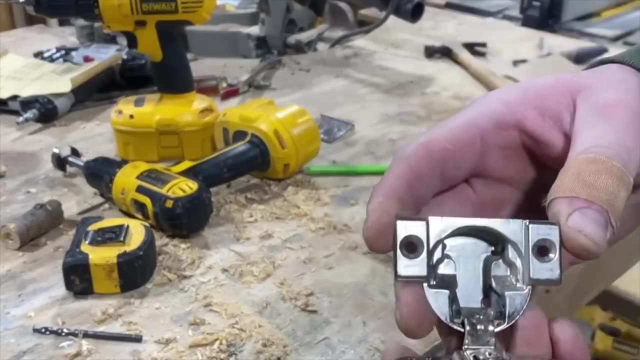 around, but 3 quarter inch material works best, And that's because in this video I give you the exact dimensions, so you don't have to use trial and error like I did. Plus, I think it's kind of cool that this thing uses a cabinet hinge so it can open and close, So once. 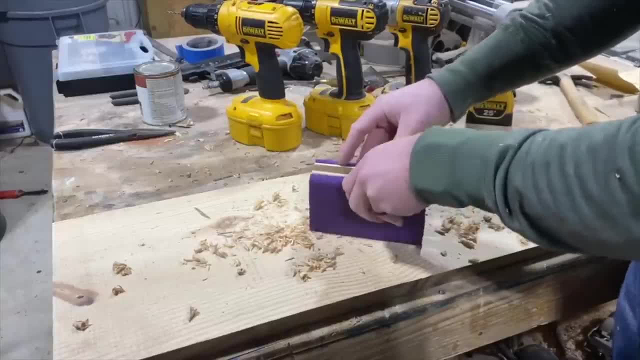 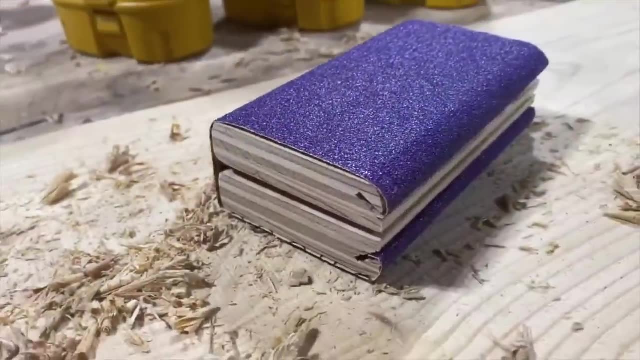 project. not only do you get experience, but you get a new tool, and who doesn't want that? And now, those tight corners are no match for this guy If you only have small pieces of scrap wood laying around and you need just a little bit of storage. 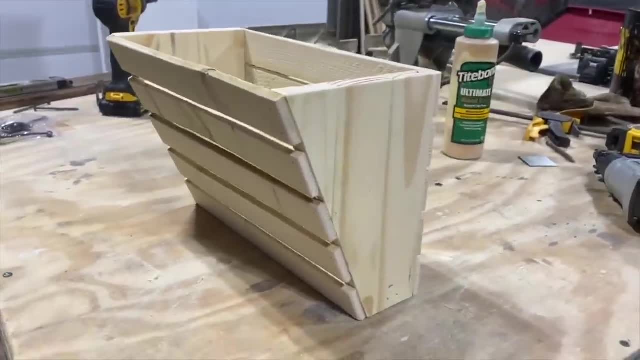 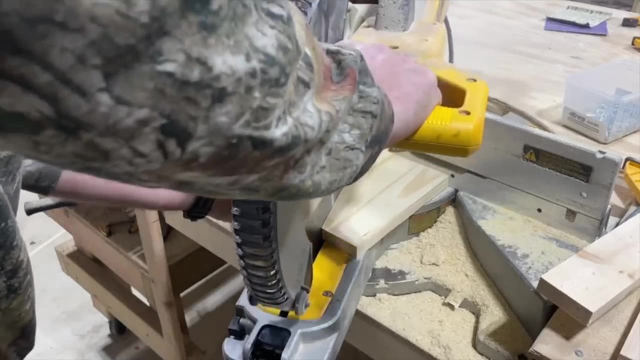 try making the hanging basket. These are really similar to the crates, but they actually hang on the wall, and these are really easy to make. Depending on the scrap wood I have laying around, I can make one of these in about 10 minutes. They're super simple, especially if you have an 18. 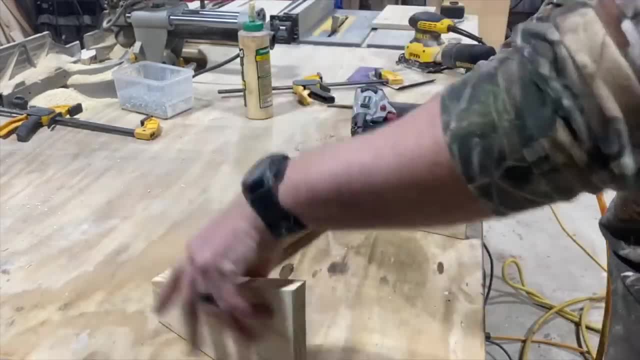 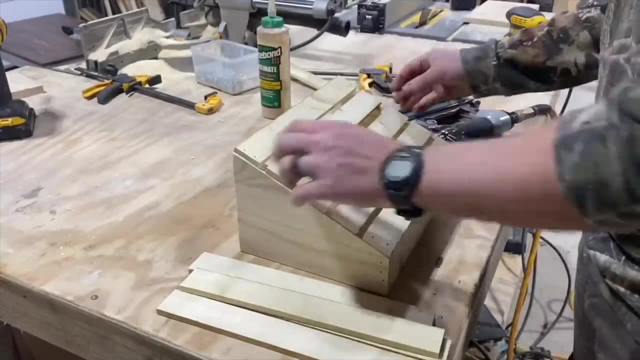 inch nailer, like I do. If you don't have one of these, no big deal Regular finishing nails work just fine. For this particular hanging basket, I actually use strips of lattice to make the sides, but you could also rip up 2x4s or other dimensional lumber to make these pieces. 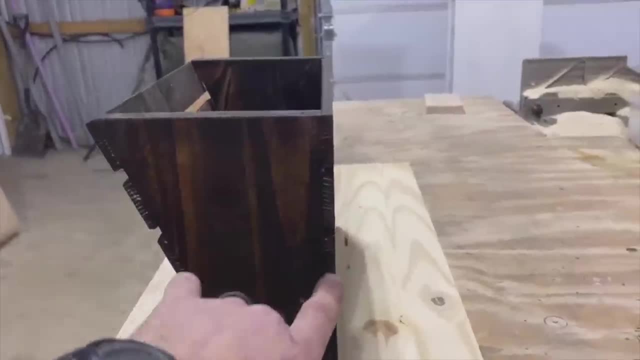 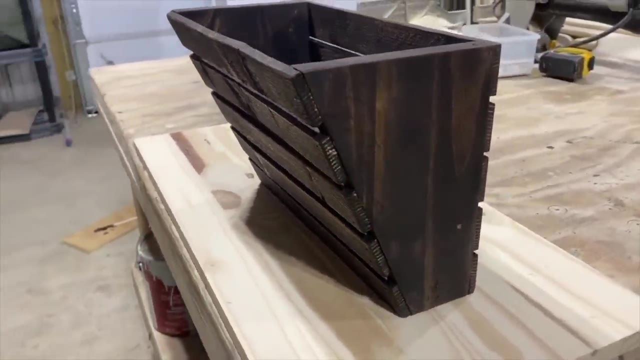 But, as you can see, these are pretty cool because this flat side allows you to hang it on the wall. Then this makes a great place to hide all your junk when company comes over, And, as you know, it's all about keeping up with appearances. Another project that's really fun to build are kids chairs. 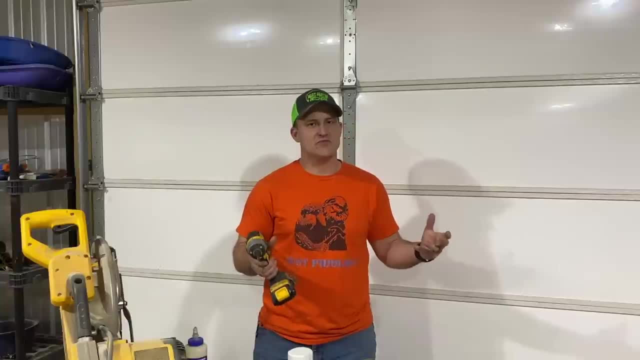 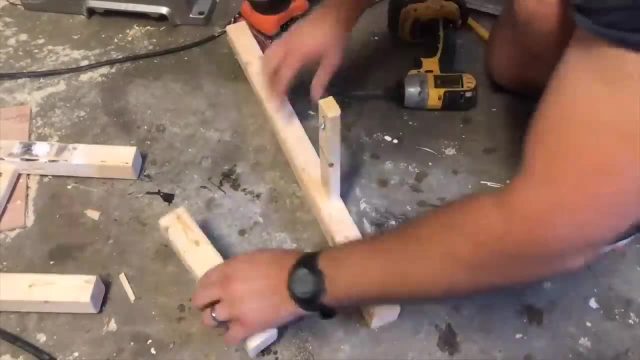 These eliminate medium-sized pieces of scrap wood and kids love them because they feel bigger than they actually are, and adults love them because the kid actually sits still for five minutes. Now, obviously there's a million different designs out there for kids chairs. This is just a simple. 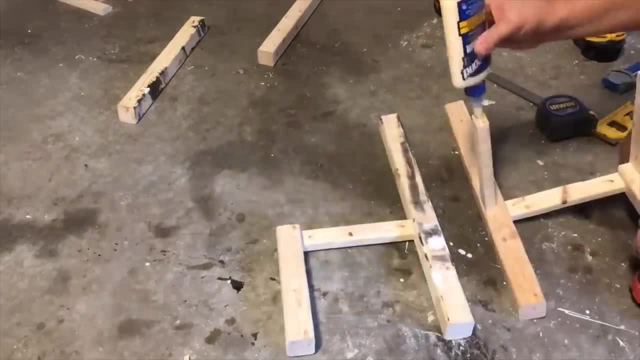 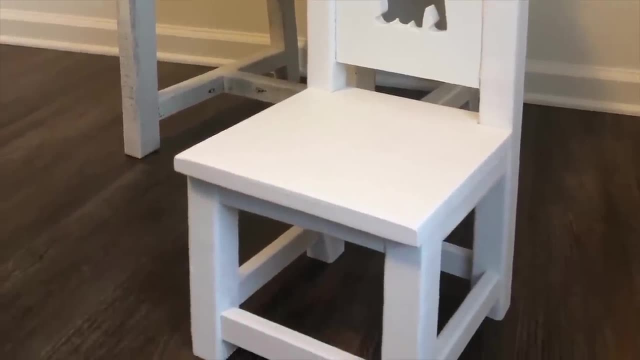 design that you can make out of scrap wood you have laying around. Think about all the scrap wood you could eliminate if you built four chairs and a table to go with it. And I don't know about you, but when I was a kid I always thought little stuff like this for my room was pretty cool. 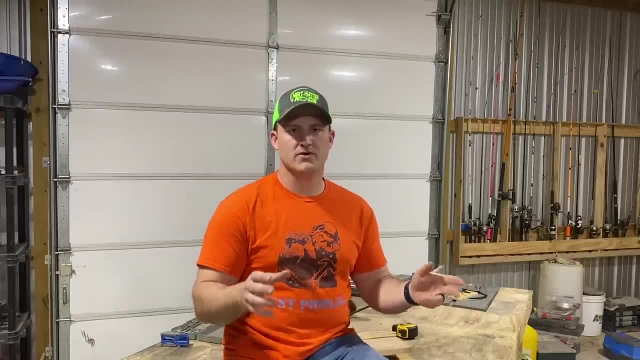 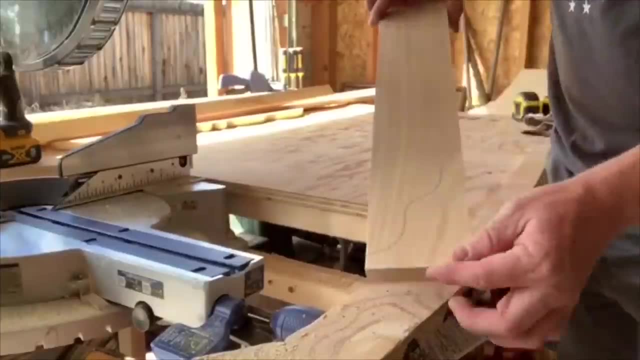 If you need more shelves somewhere, don't go waste money at Lowe's or Home Depot on shelf racks. Build yourself some corbels instead. These are a great way to eliminate that scrap wood Now. I built a lot of corbels over the years. 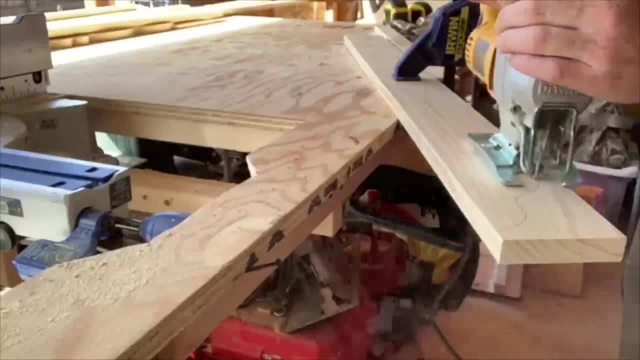 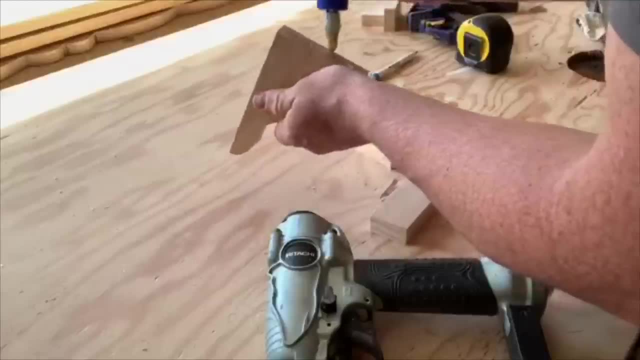 but this particular video was made by my brother-in-law, So it just proves the point that not only are these easy to make, but there's about a million different ways you can make them. And who couldn't use just a few more shelves in their house? And you do the math If these 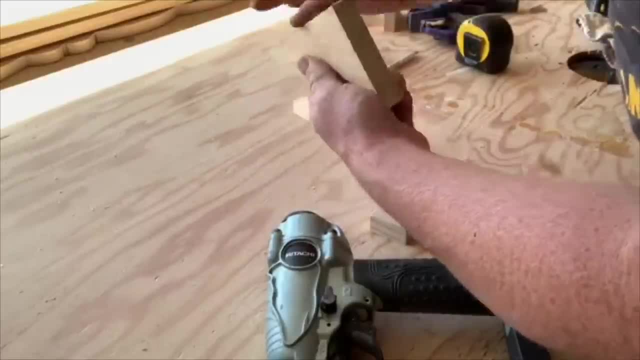 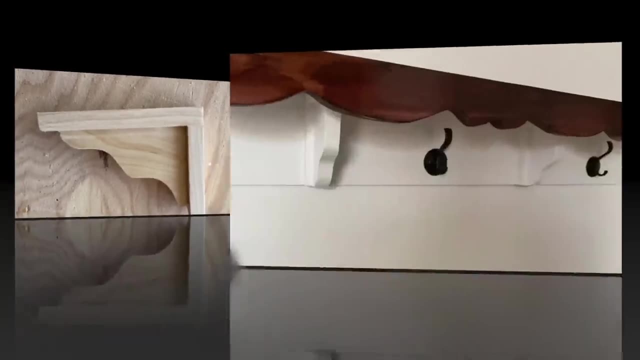 things are like five dollars at Lowe's or Home Depot and you're going to be putting a lot of shelves in your house. this could save you a lot of money if you just build these corbels yourself, So you can easily make a lot of these from the scrap wood you have laying around. 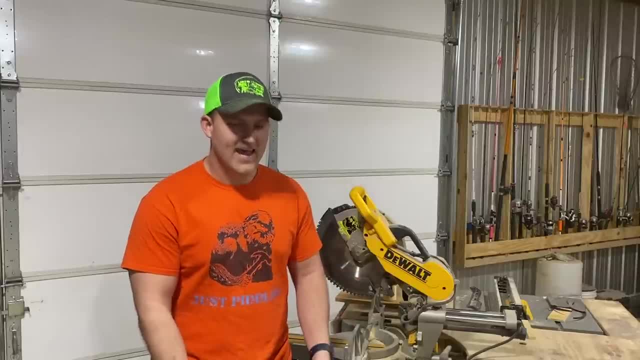 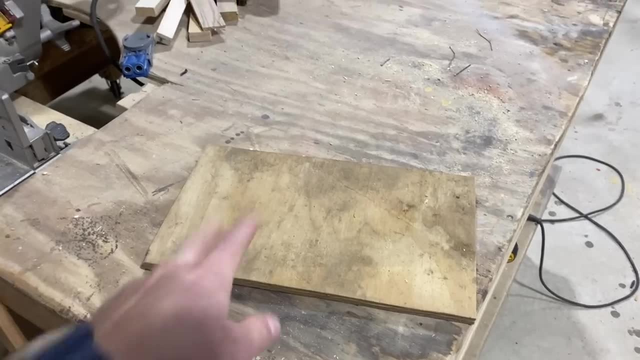 Now for a scrap wood project that makes the perfect gift idea. Handmade cutting boards like this make the perfect gift for Christmas, birthdays and even Valentine's Day. I gave this cutting board to my wife for Valentine's Day about two years ago and it was such a hit that 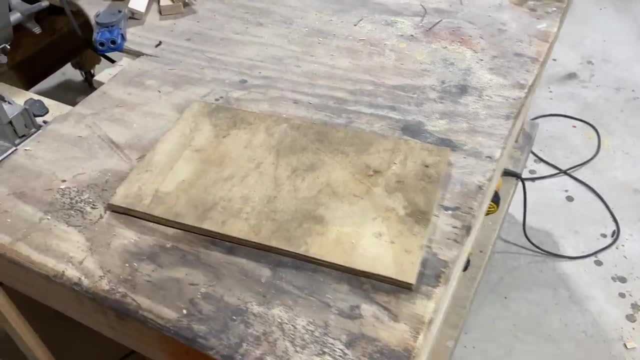 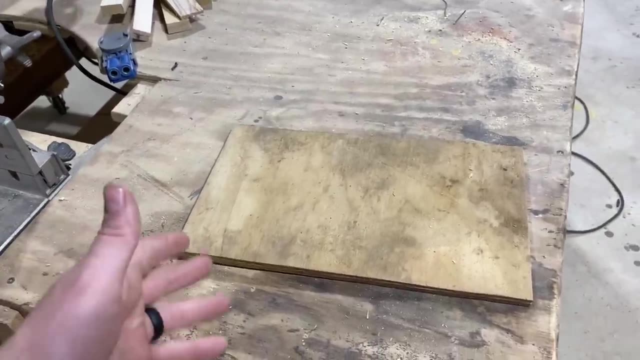 she hasn't asked for another Valentine's Day gift since And I knew it was going to be a hit because I've laid a nice big bass on it and it worked super well and I knew she was going to be excited it up for wrapped it up and it was a perfect gift, or you know, if you have. 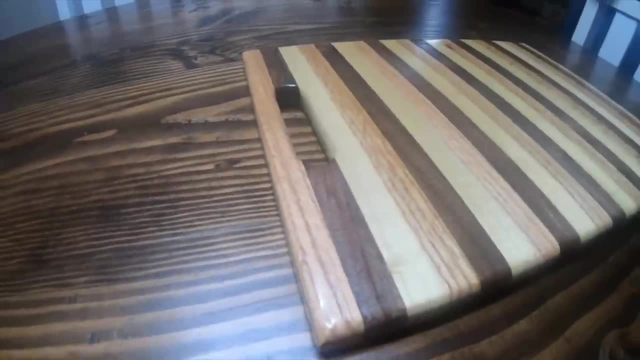 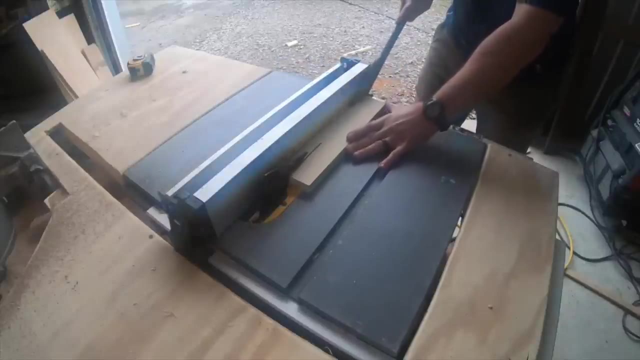 scrap hardwood laying around. that works too, and you know, cutting boards are pretty easy to make, especially if you have some kind of planer. but if you don't have a planer, this particular design is made so you don't need one. I know that's probably the biggest limiting factor when you're first 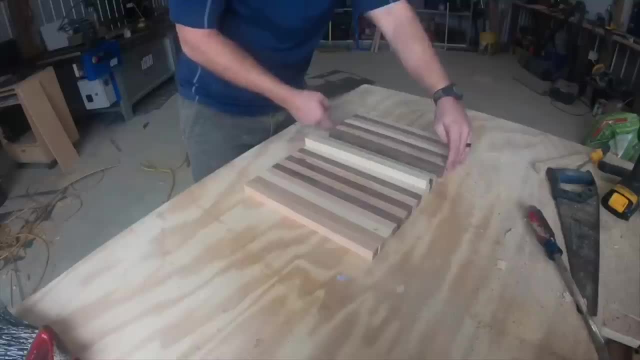 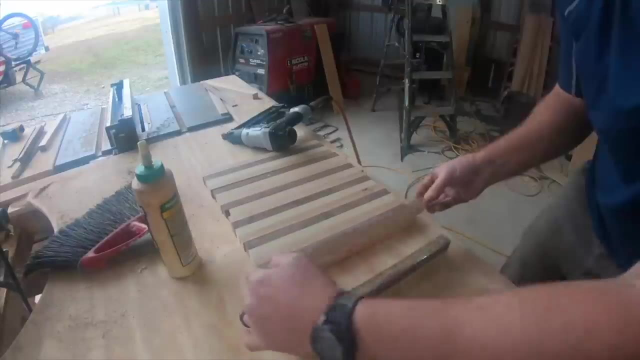 getting started. you don't have a lot of the tools you need to make certain things, and this particular video will help eliminate that problem. and even now I actually only have an electric hand planer, so I kind of prefer this method for making cutting boards. if you do decide to watch this video, just ignore. 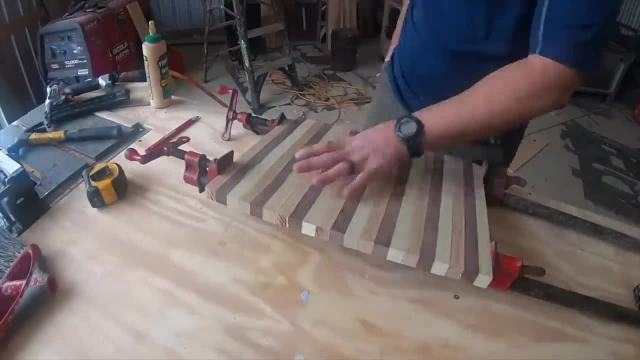 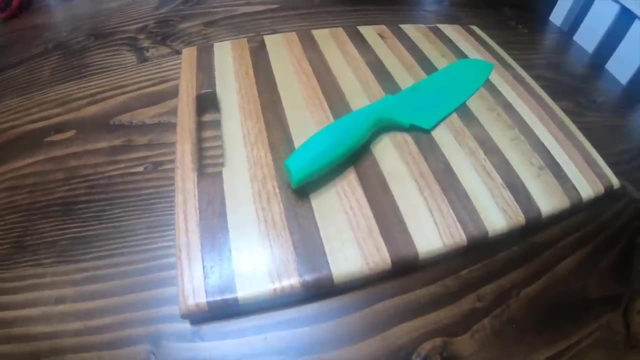 the fact that I could have used a little bit better wood to make this thing. I just used the scrap wood that I had laying around and it still made a perfect gift, and it's still going strong today. I think it turned out pretty decent for just a bunch of scrap wood, don't you? especially since I don't know? 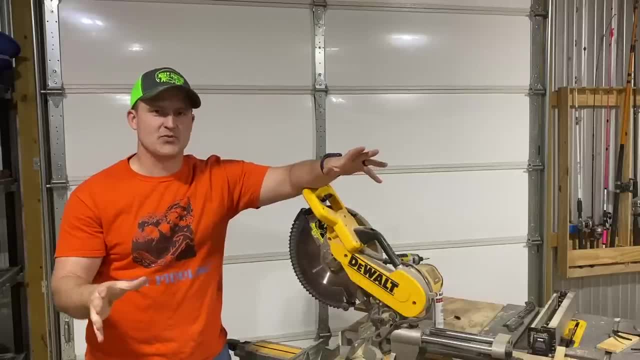 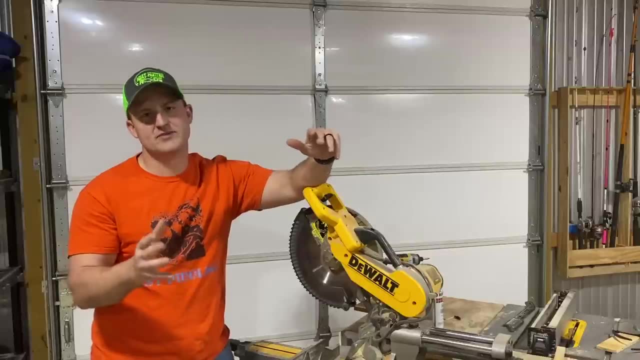 what I'm doing now for the tenth and final scrap wood project I have for you today is toy logs. this one is a really cool project if they're not really that hard to build. they're a little bit time-consuming, but they're a lot of fun. 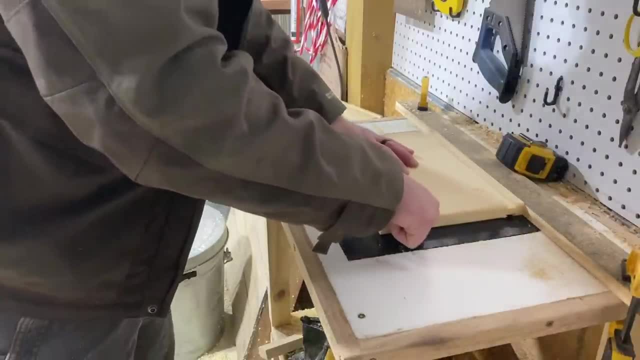 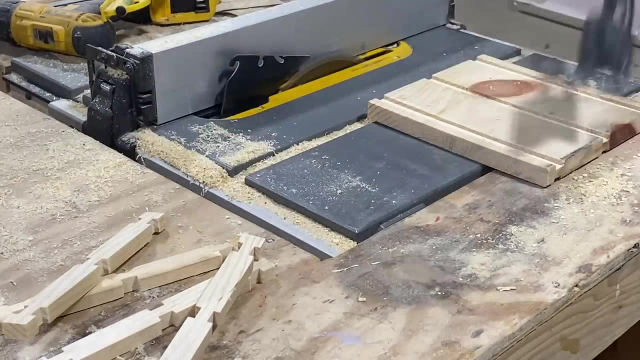 and I hope you enjoyed this video and I'll see you in the next one. and the kids love them. this particular design uses 3 quarter inch material, because that's what I had most of laying around. I also wanted to eliminate as much routering as possible. to save a little bit of time, I made all these.